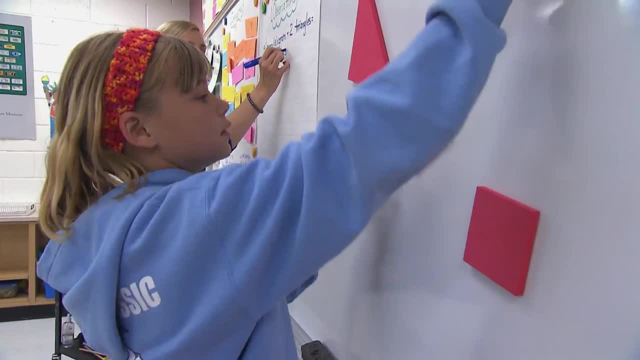 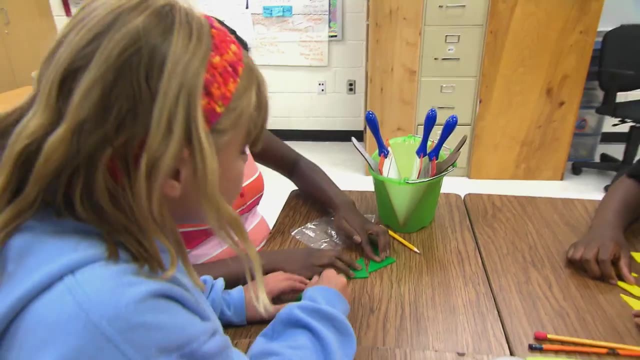 It just allows me to see what they're thinking. It also, when you let them be open-ended like that, it gives you an idea of what kind of math is on their brain. I know you can't, but Make it on, Make these into squares. 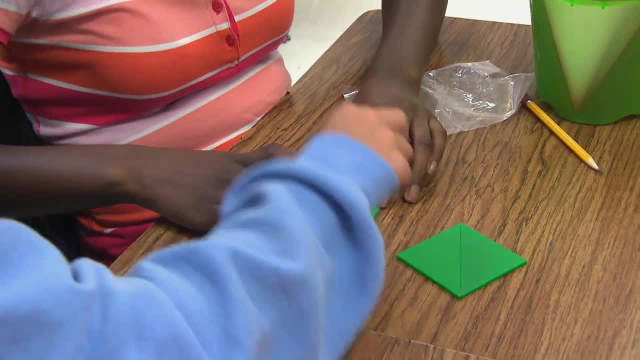 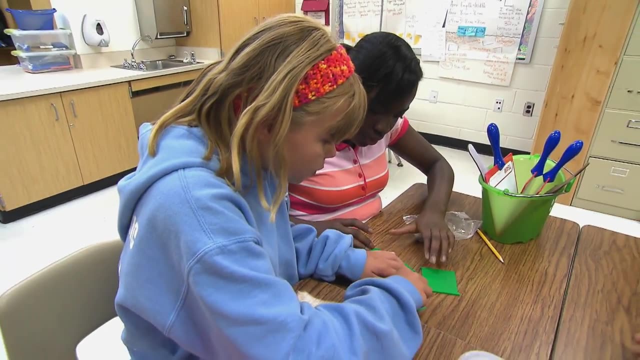 We make these into squares. We can put some of the ads because of this one. We just need to figure out a way to make them into squares Or rectangles. Oh, we did it. We did it, Something that should be really important to us. 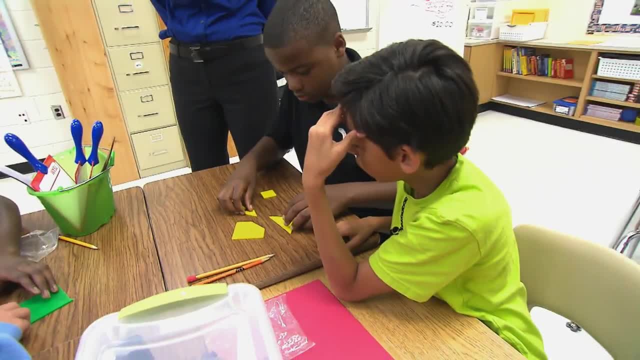 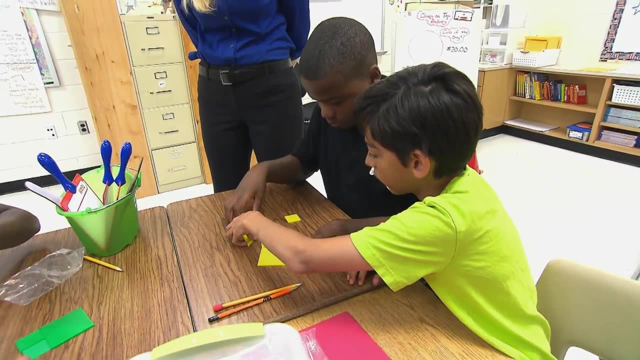 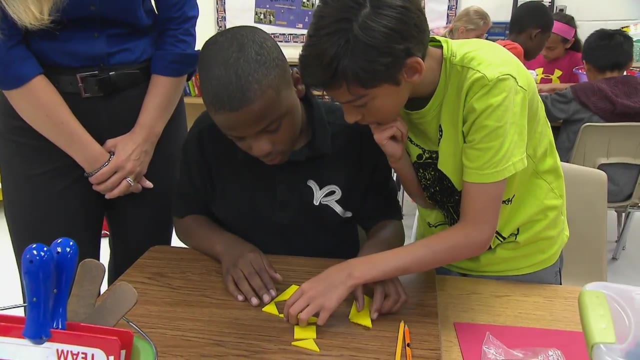 as math teachers is students generating math talk. So by working with a partner, that person is their sounding board. That person often creates an atmosphere where I'm more comfortable saying this because it's with my peers. so I'm gonna try this idea out on this person. 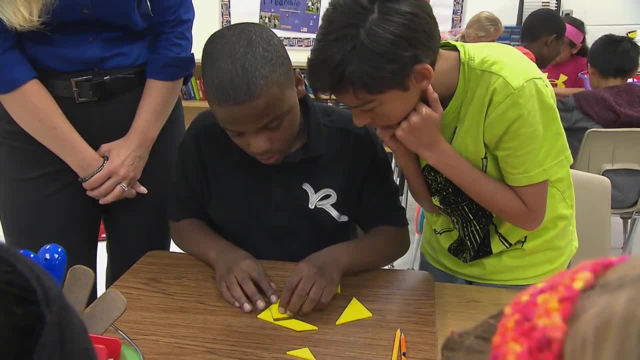 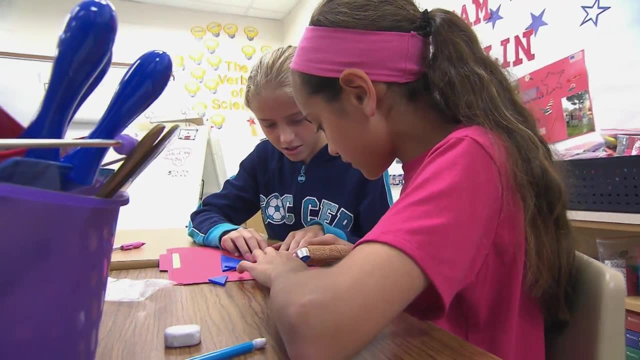 And depending on what they say back, it'll kind of validate my idea. Keep your paddle up if you'd like to explain your thinking. I also believe in scaffolding the student talk. So they started in pairs, But then the activity then led. 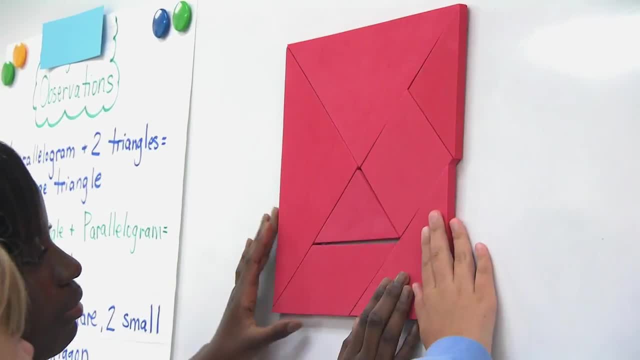 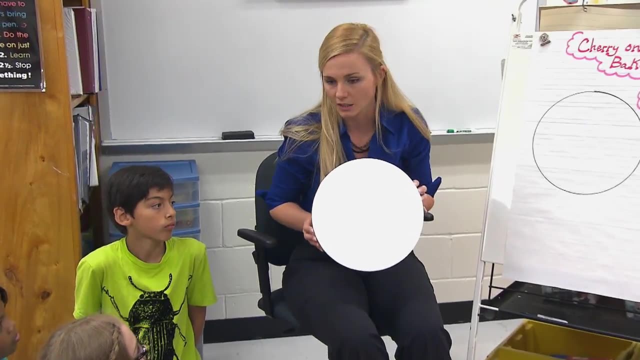 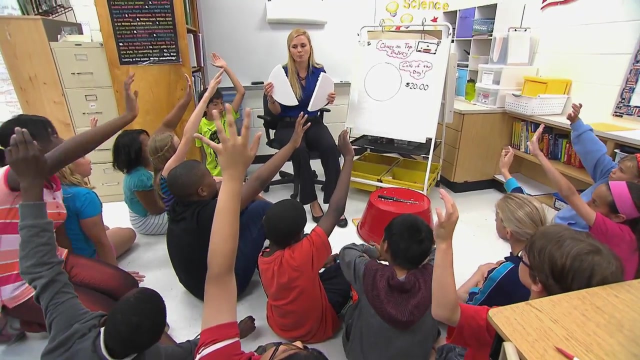 to more of a whole-group discussion, where small groups or even individuals were sharing an idea that was created with another person. And then I took that model, that concrete model, and I changed it a little bit to a circular cake and I cut the cake into fractional parts. 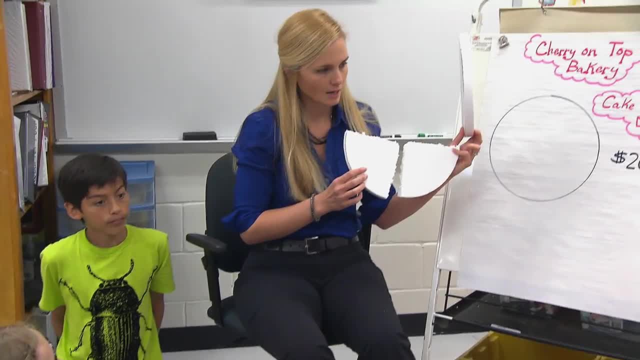 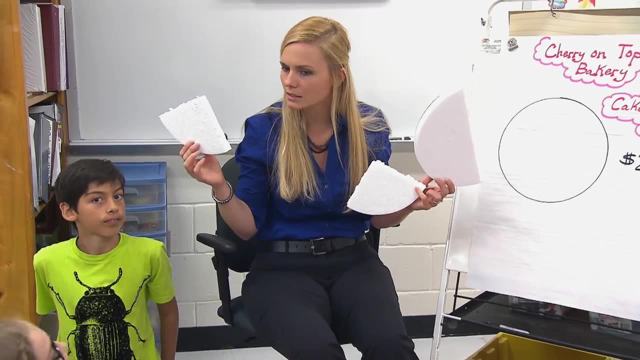 And we assigned an amount of money to each piece of the fractional part. Are you thinking in your head right now what fraction, What fraction of my whole cake this represents? Are you thinking in your head? I know how much that piece of cake would cost. 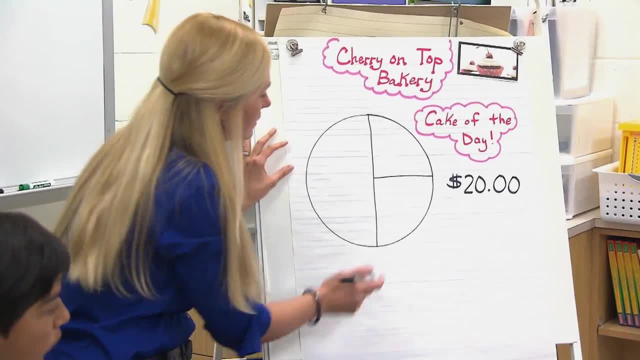 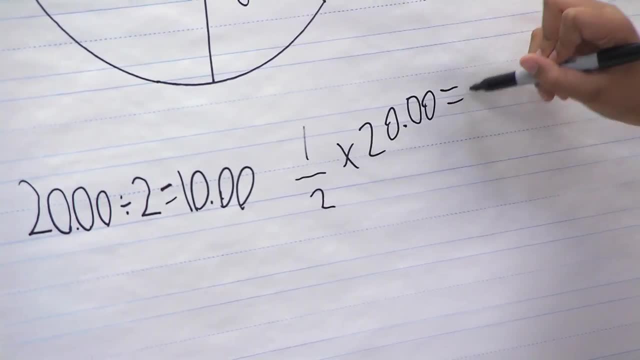 Although it's real-world math, it's abstract to them, because how do you get from there's this piece of cake to this piece of cake costs $5? So students need to be able to see it, and that's where modeling is so important. 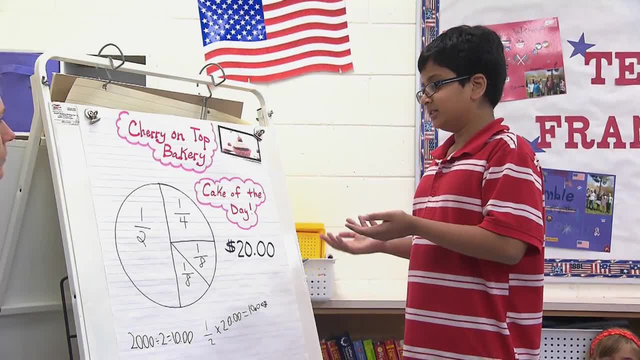 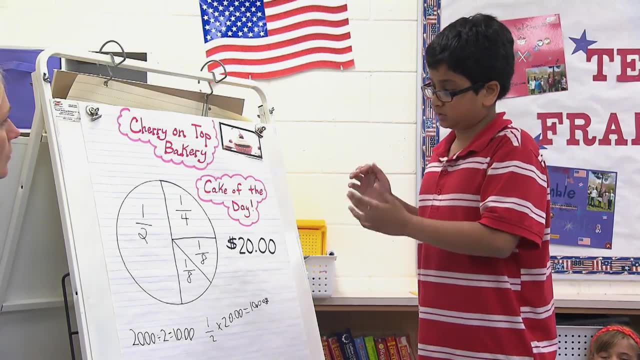 One times 20 would equal 20,, of course. but then if I did half, which is half of 1,, then you would also put half of 20,, which is equal to 10.. Okay so, when you say 1 half times 20,. 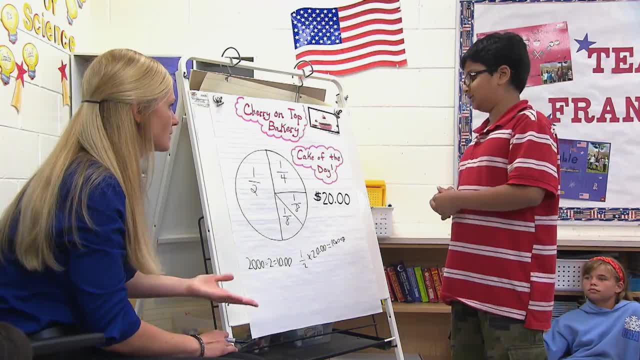 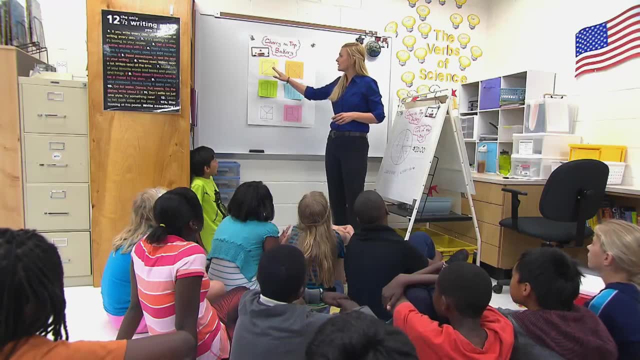 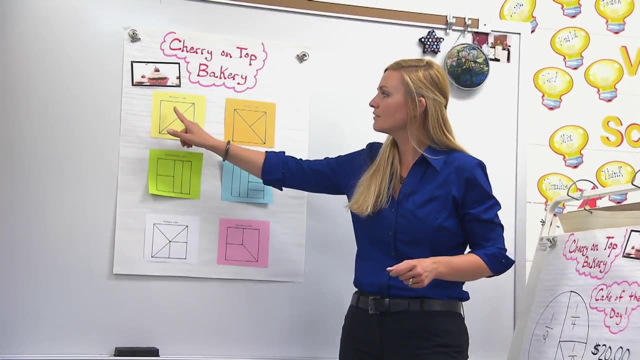 it's like saying half of 20 is equal to $10. Excellent. We then moved away from a concrete model and students were given pictorial models of different cakes. Your task, with your partner, is going to be to see if you can find the cost of each piece of cake. 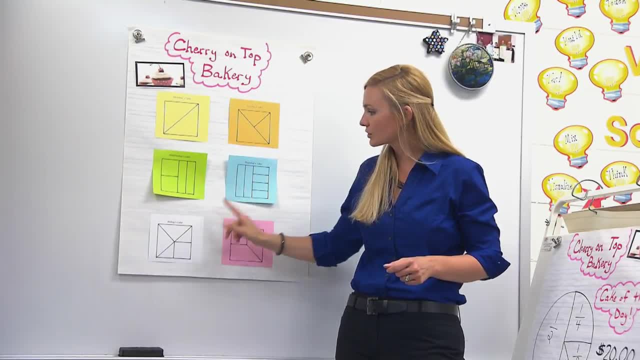 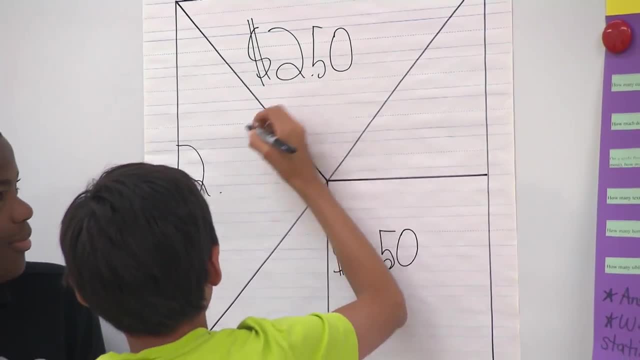 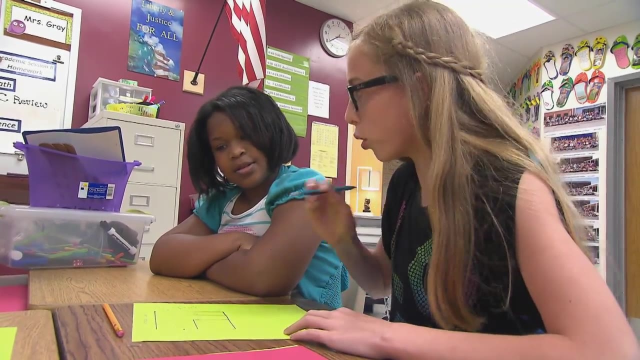 for Monday, Tuesday, Wednesday, Thursday, Friday and Saturday's cake. And it's once we get to the number representation that we really can understand what students have gotten out of the math, Because each piece of cake is 1 fourth of the whole cake. 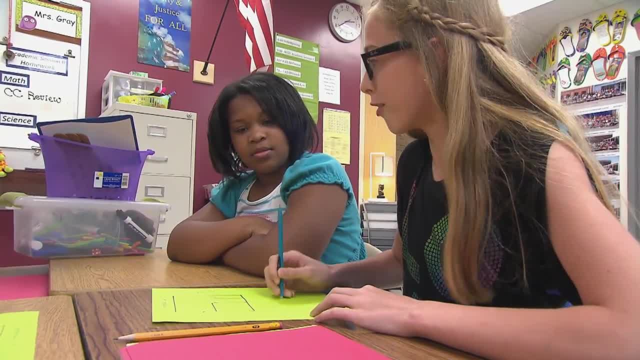 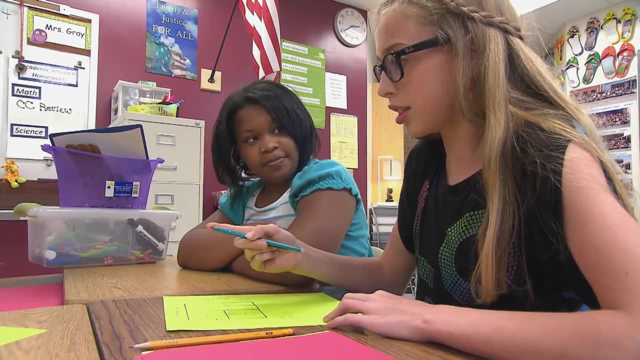 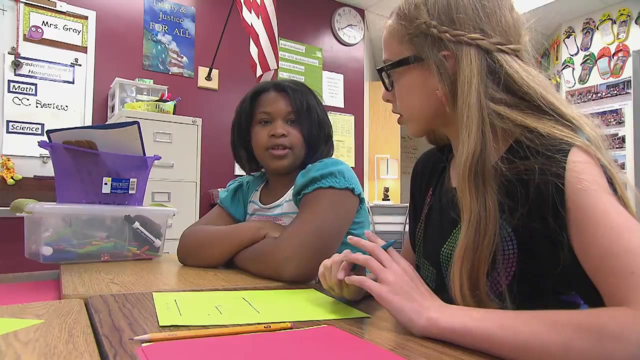 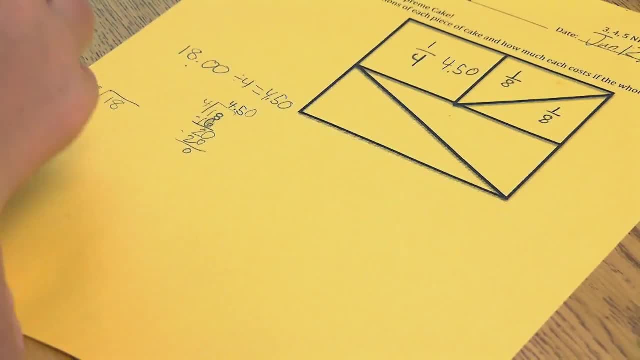 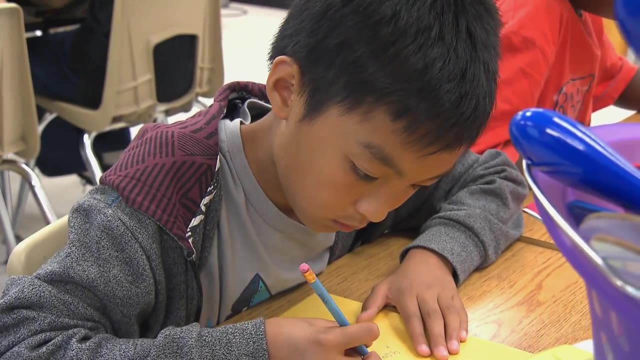 The exit ticket at the end was another cake. It was a square cake cut into various sized pieces. I'll use that exit ticket as a formative assessment piece to let me know who has understood how to find part of a whole when the whole is not one. 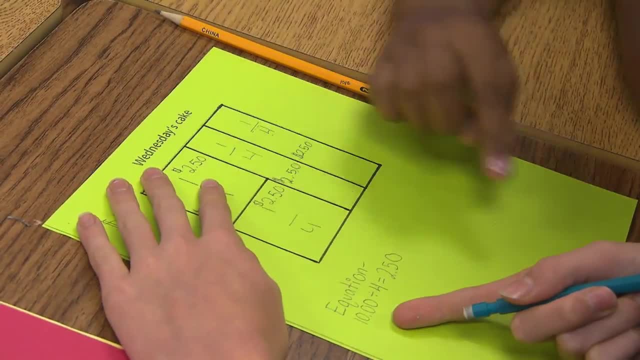 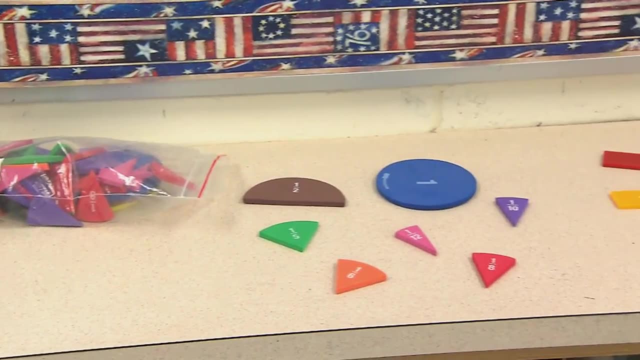 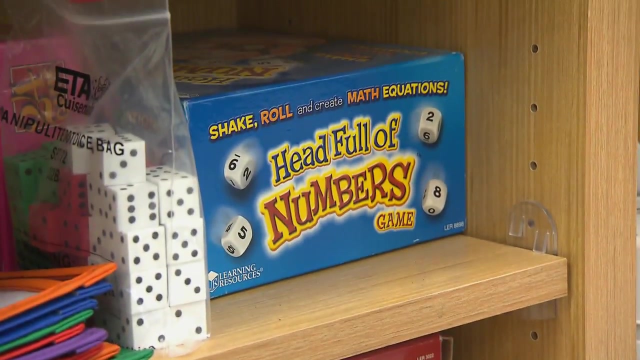 and who's able to use a number representation or a number model for that. As math educators, we need to know that we're not going to use the same fraction model every day. Using the various models allows us to reach all of the learners, versus this one model that might work really well. 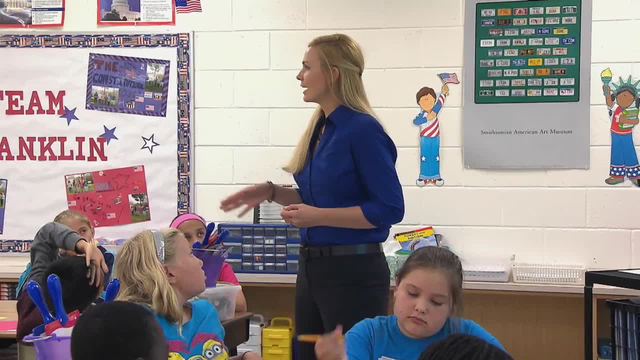 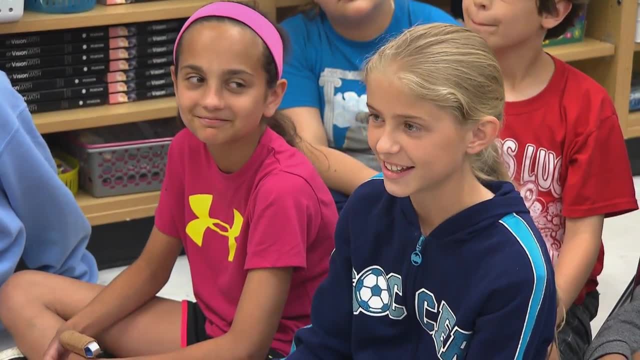 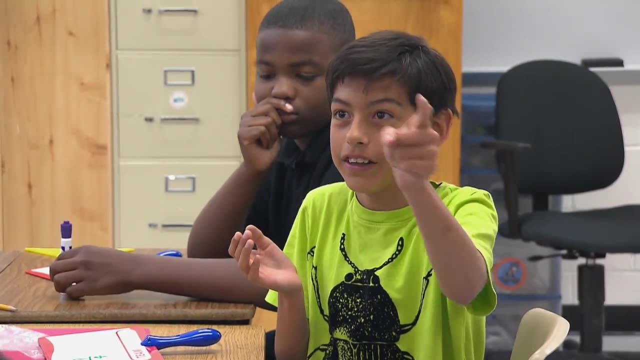 for this 10 kids. By varying the model, we ensure that all students are learning the math. This idea that math is everywhere is really a critical focus for us as educators. If we want students to enter fields in STEM, we need to help them see that math is everywhere. 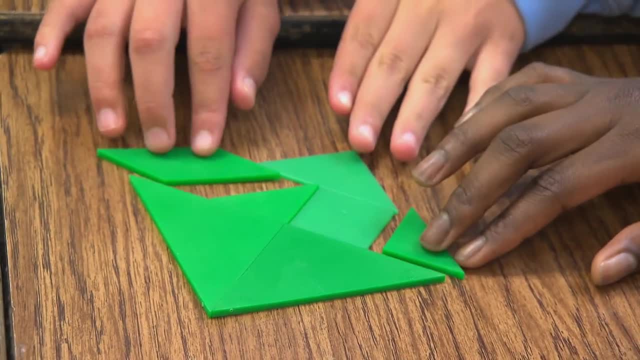 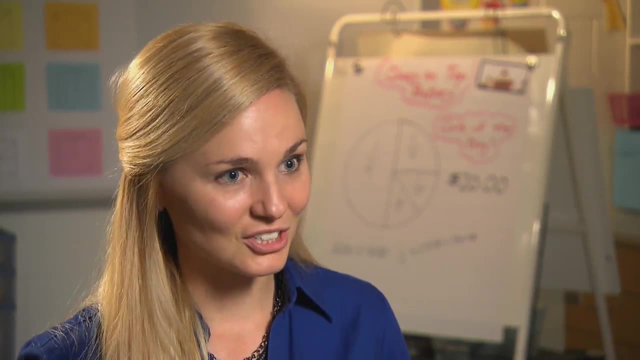 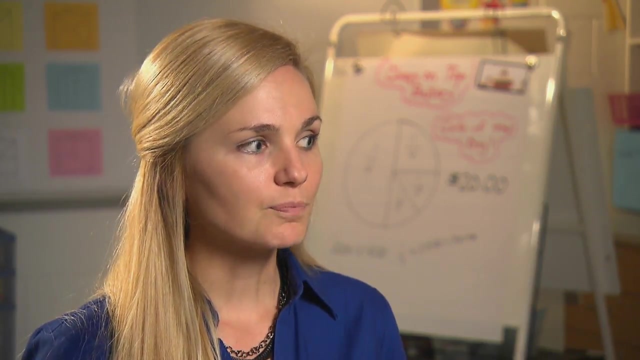 and everybody can do math. So this would probably, This would go here and here: Hooray, So that as they enter sixth grade math and then one day enter ninth grade math and college math and math becomes more abstract and possibly less contextual. 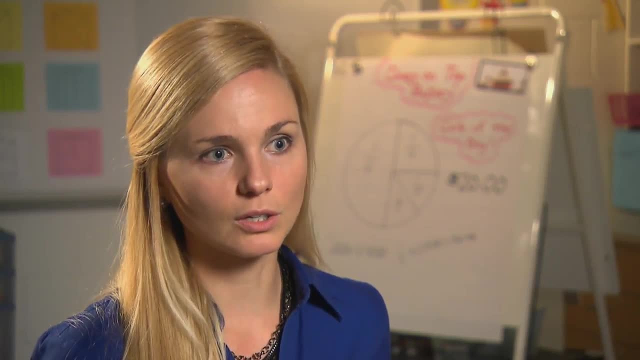 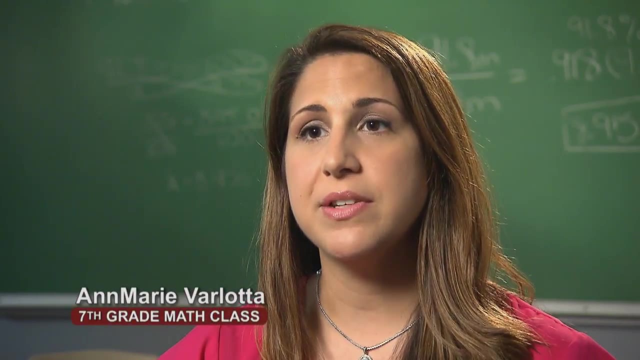 they have these models that they remember from early on, working with fractions to connect to. In this lesson, modeling is a really important factor, because we're taking a real-world problem and we're applying math to it, And so we're modeling with mathematics. 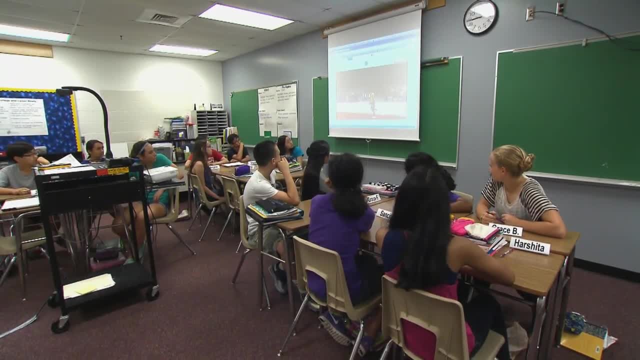 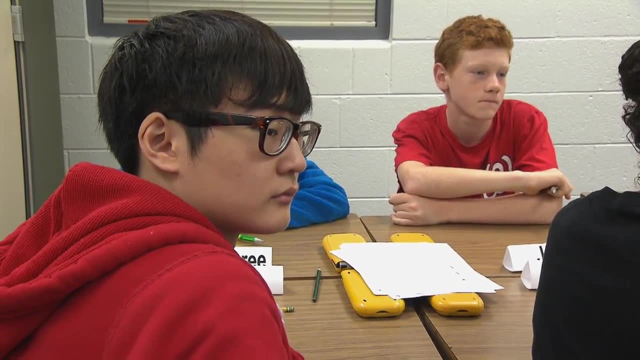 based off a real-world application. The students first looked at a video from the 2012 London Olympics of the 100-meter dash. I just asked them what they noticed about the video, because it's really When you're just watching the video or you're looking at the Olympics. 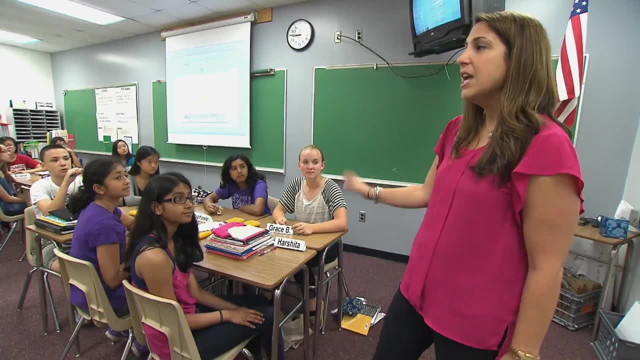 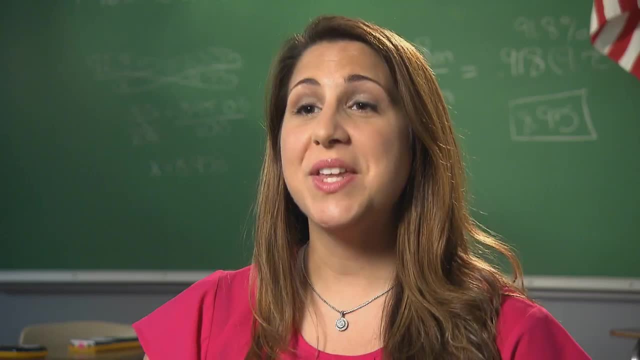 you're not thinking about the math, that's there, But there is math. Is there any math in this video? The probability or chance of someone winning the race. So then I put up a picture of the three winners, and it's clear that Usain Bolt is taller. 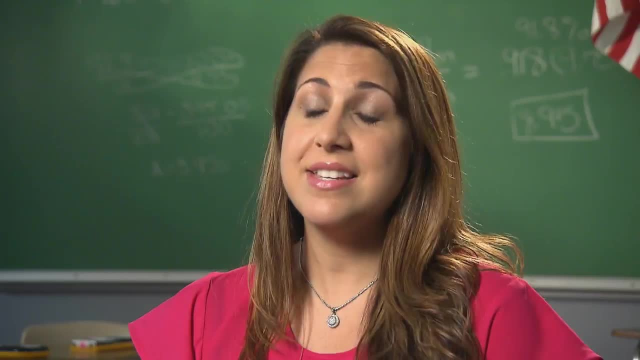 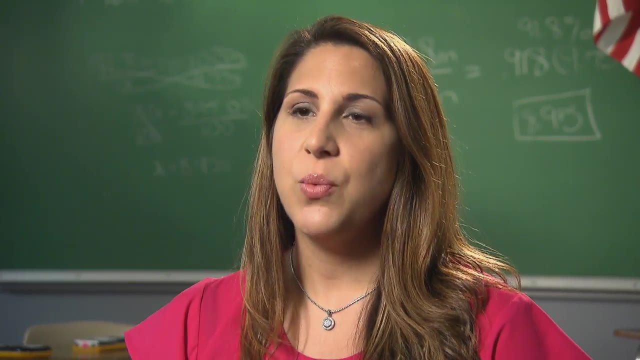 than the other two sprinters. And so the question naturally arises: did he win because of his height? Does he have an unfair advantage because he's taller? And so the students think that that is the case. and then we start to think about: well, 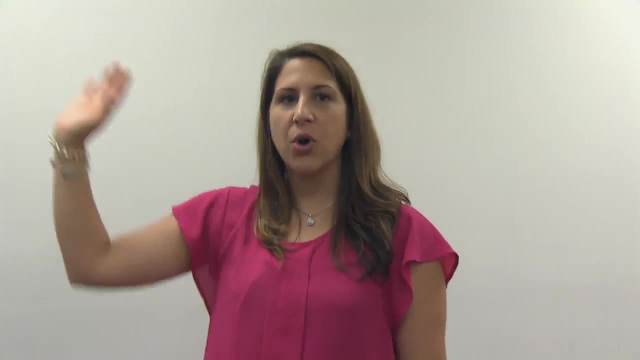 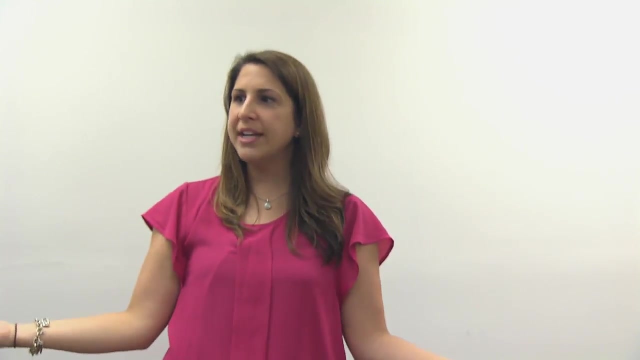 is there a way to figure that out? Raise your hand if you think that being tall would give you an advantage in sprinting. Well, that's a majority. Look at that. Almost every hand is raised. Why? Why do you think that being tall would give you an advantage? 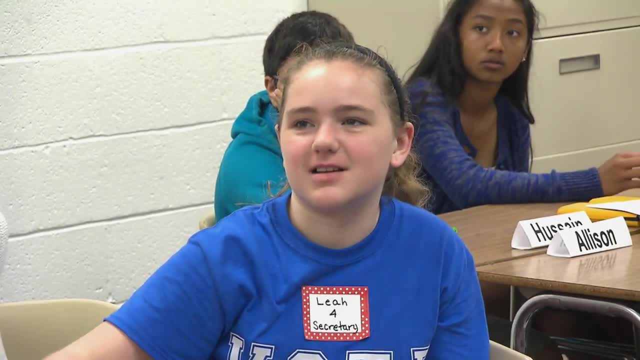 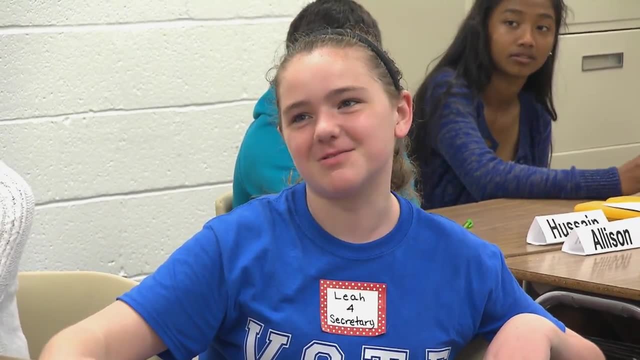 if you're sprinting a distance, We could test it out and see who wins. Like if we tested this class, we could see who the tallest is and who would win. You can use like past statistics of people that might have been like the same height. 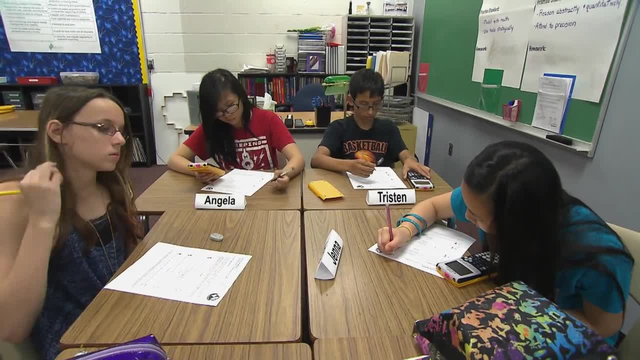 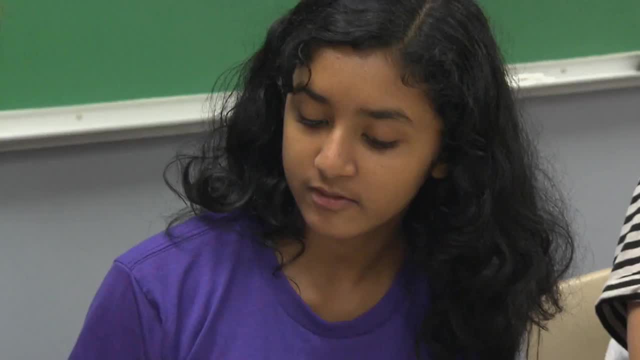 We really want the students to think about what math could work here and what method could I use. In this particular lesson, students were starting out with ratios and that was their initial model. Can we set up a proportion? A proportion would be a really good idea. 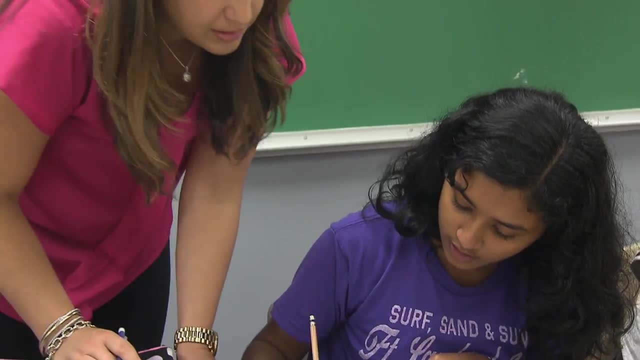 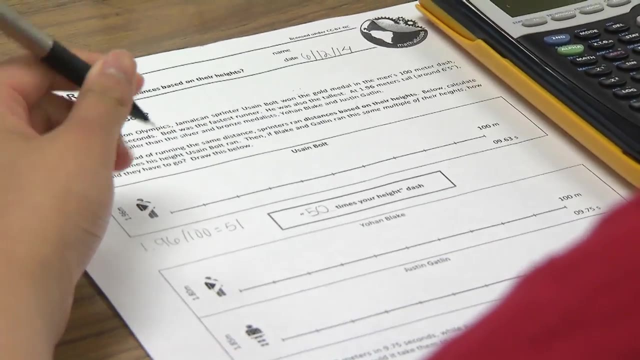 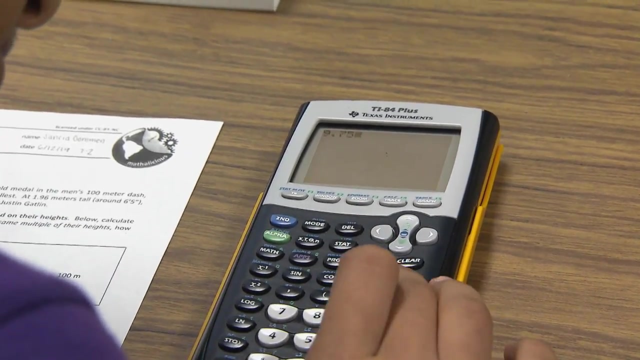 What would that look like? 100 meters per the 100 meters time. Some students turned it into a proportion. Some students did it a little differently. Some students looked at it in terms of running a percentage of what they ran overall. We're formulating a problem and then we're 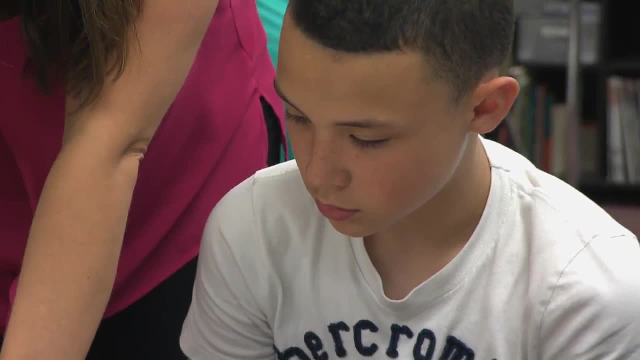 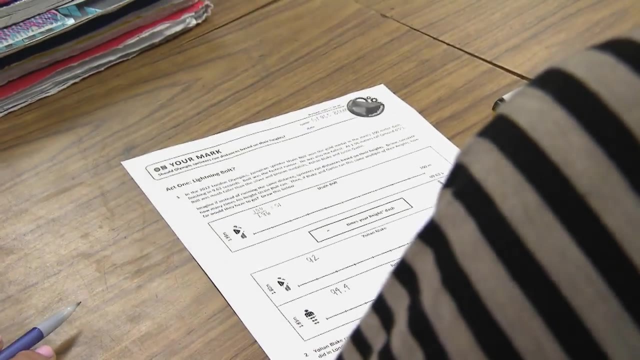 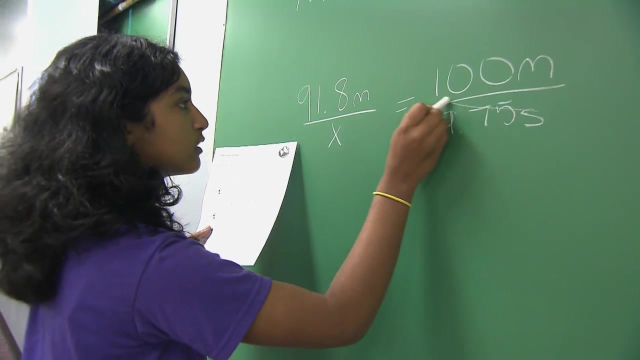 creating a mathematical model to analyze and support a conclusion that may or may not work, And sometimes with modeling, you may start on a path that makes sense, but then you have to reanalyze the model that you apply to, whatever the problem is or the math that you're using. 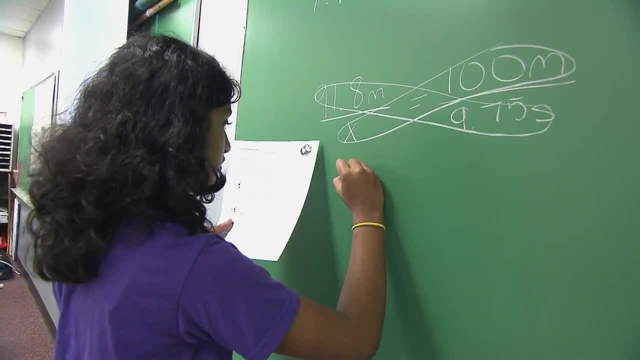 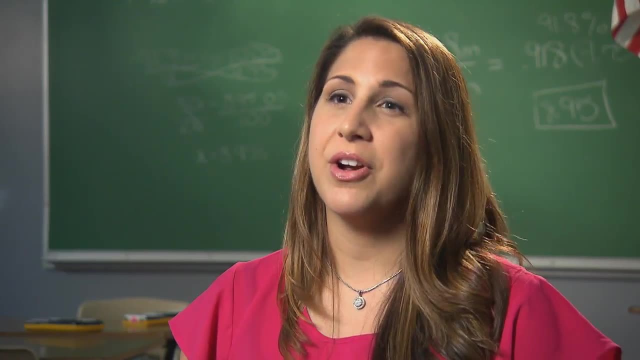 And you may have to make adjustments, and that's okay too. That's all part of mathematical modeling. I'm listening for them to think about the problem in terms that they are comfortable with. What do we need to do to this number?